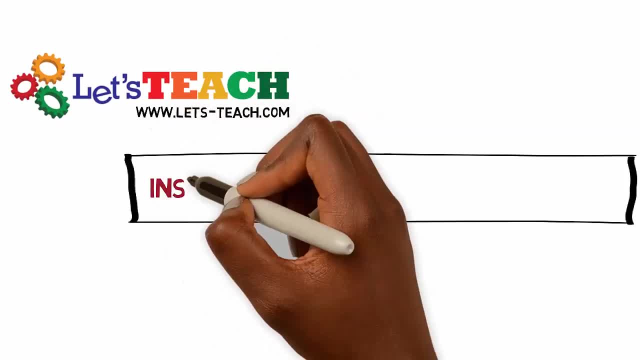 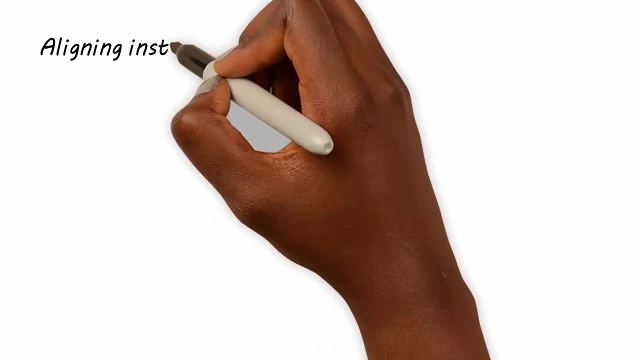 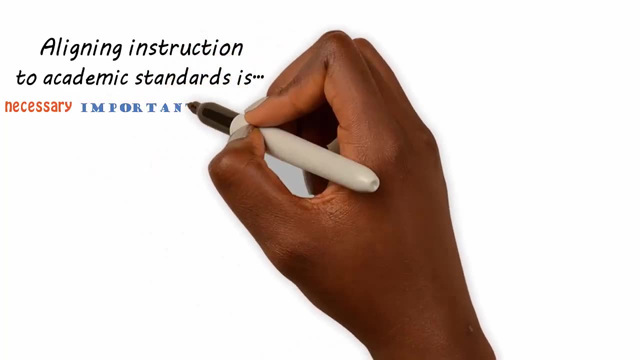 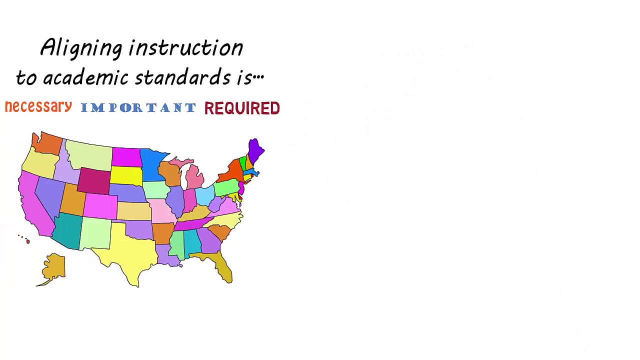 No matter what grade level or subject you teach. as teachers, we are all bound by at least one expectation: By law: we must teach our state's academic standards. While most states adopted the Common Core standards, eight states chose not to. Regardless of that, 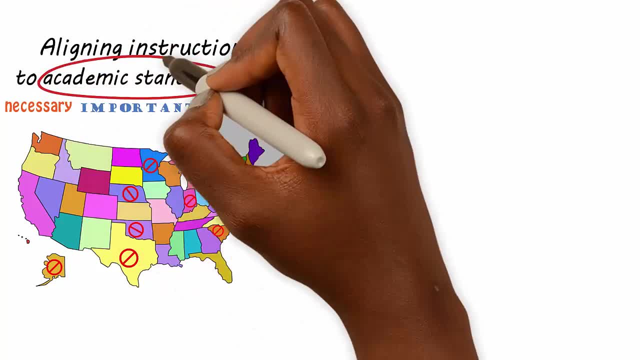 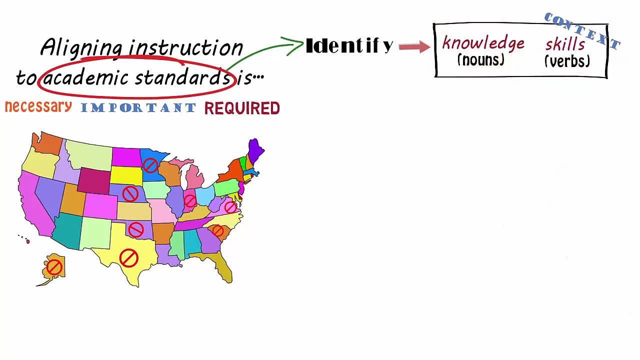 fact, all academic standards are constructed the same way. They all identify what students must know and be able to do within a certain context. For example, take a look at this 5th grade mathematics standard. It expects students to compare and order two decimals to the thousands and represent comparisons using the symbols. 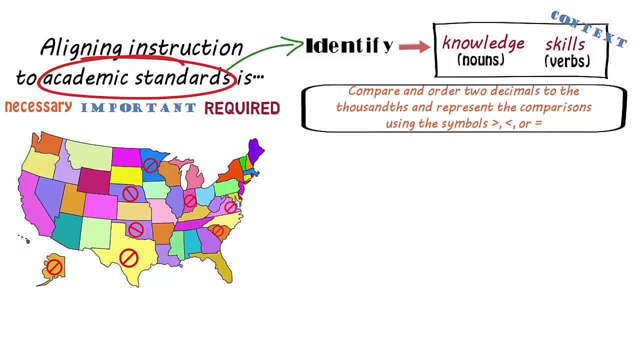 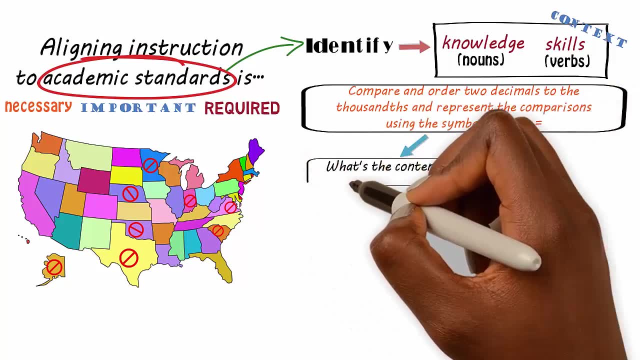 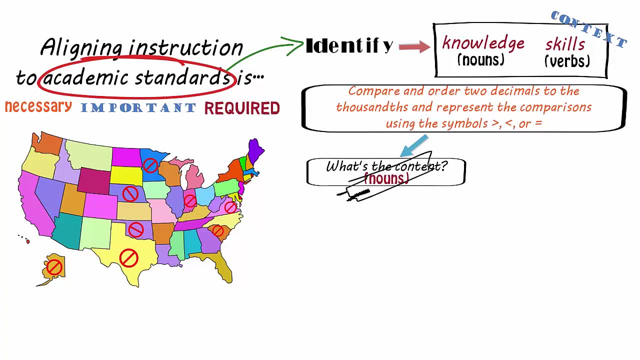 greater than, less than or equal to. The first thing we need to figure out about this standard is the content that's being addressed. What do students actually need to know here? Well, most nouns in any academic standard will help us identify the content. 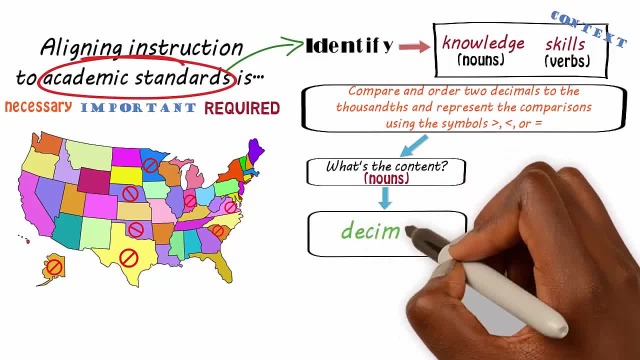 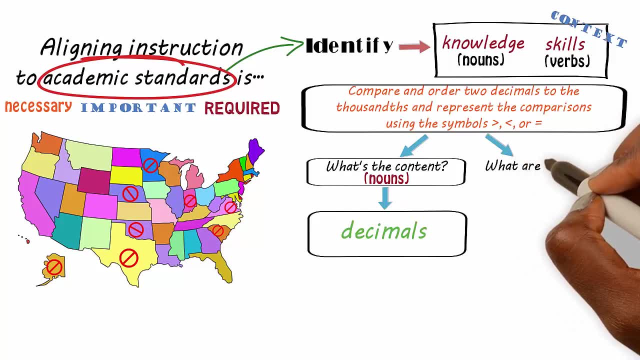 so in this case, we'll need to teach decimals. The next question is: what skills do students need to learn? We'll use the verbs and verb phrases found in the standard to answer this question, So students will need to compare order and represent comparisons of decimals. Finally, 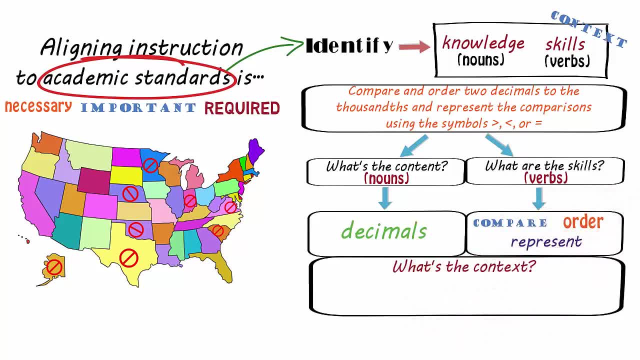 we need to identify the context, and in this case, students have to represent comparisons using symbols, and the comparisons are to be made up to the thousandths place. Now it's important to note that context can also be implied in academic standards. In this example, 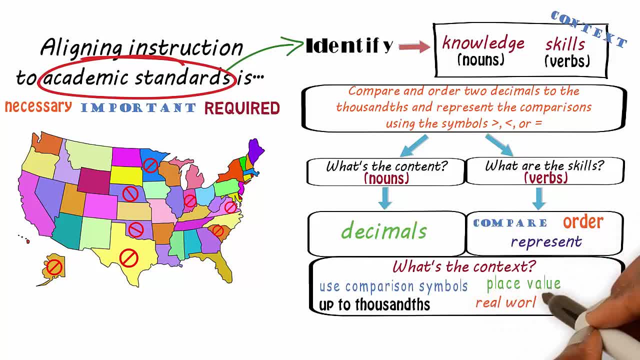 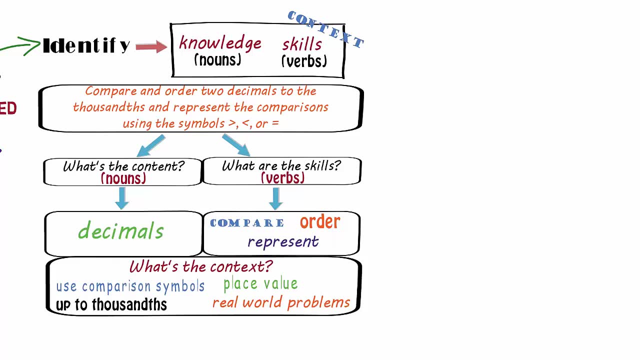 place value and real-world problem situations are the implied contexts within which students will compare and order decimals to the thousandths. As you can see, unpacking a learning standard is not an overly complicated process, and now that we understand the expectations of this standard, we can begin to develop our 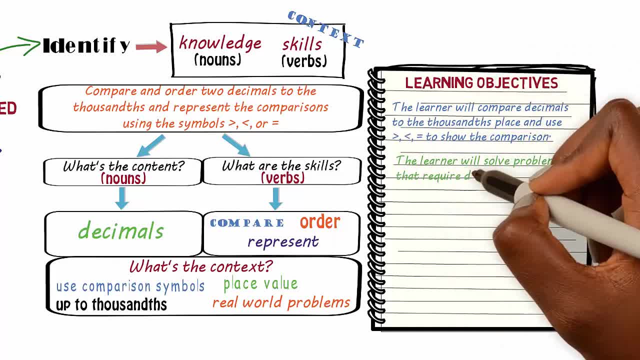 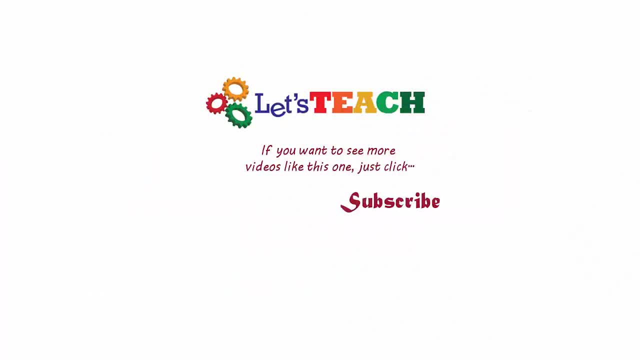 learning objectives and start the lesson planning and preparation process. See you later.